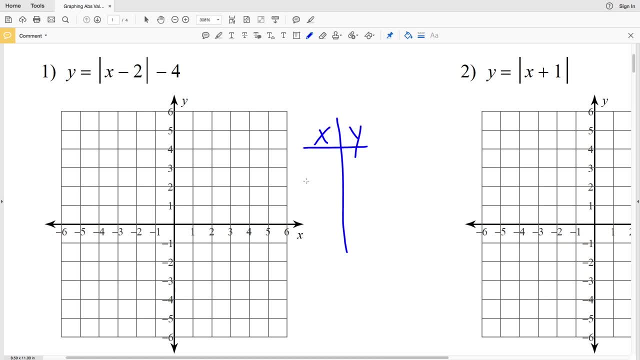 these functions- Absolute value functions- have a turning point. that's known as the vertex, and it's either a minimum or a maximum, more specifically. So let's ignore this equation for a second and think about: y equals the absolute value of x, So when we're 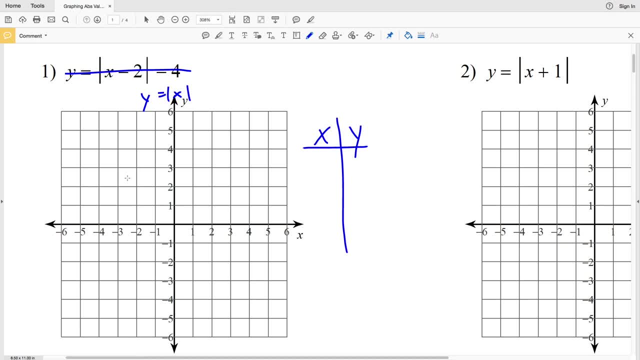 y equals the absolute value of x. if you have negative 3, the absolute value of negative 3 is equal to a positive 3.. So negative 3 in the x direction, positive 3 in the y direction, Same with negative 2- it's going to be a positive 2.. So the absolute value of negative 2 is positive 2.. 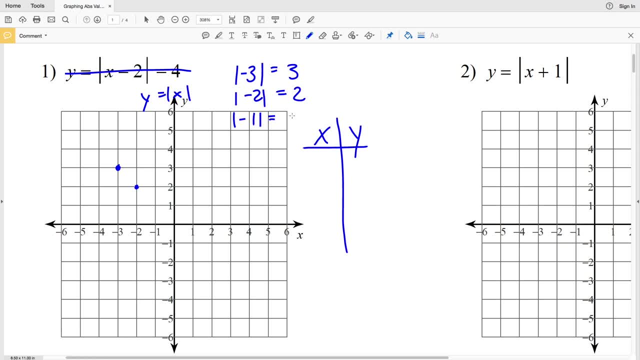 Continuing on to negative 1, the absolute value of negative 1 is a positive 1.. Then the absolute value of 0 is a positive 1.. And then we'll get into positive 1, so the absolute value of positive 1 is a positive 1.. 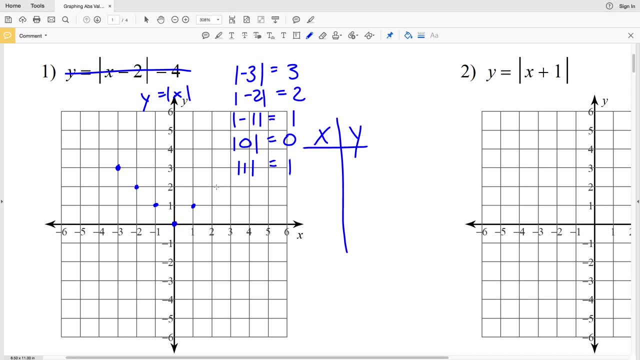 And so on. we know that absolute value of 2 will be 2.. Absolute value of 3 will be positive 3.. So you can see the turning point occurs when that absolute value was equal to 0. So it's a straight line until the turning point and then it's a straight line past the turning point. So 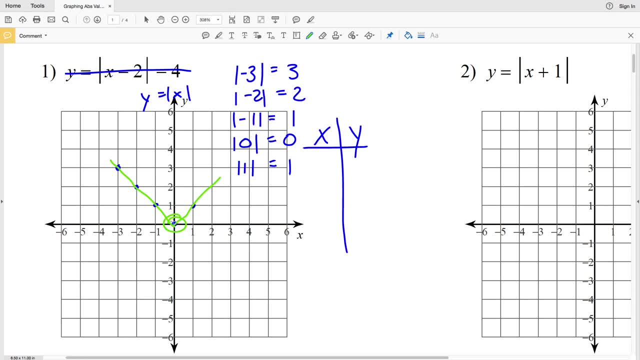 we have a negative slope and then immediately we have a positive slope, and all of that changes at that point: 0- 0. So the turning point occurs when the absolute value is equal to 0. That's true for all of the linear absolute value functions. So, in order to graph this function, 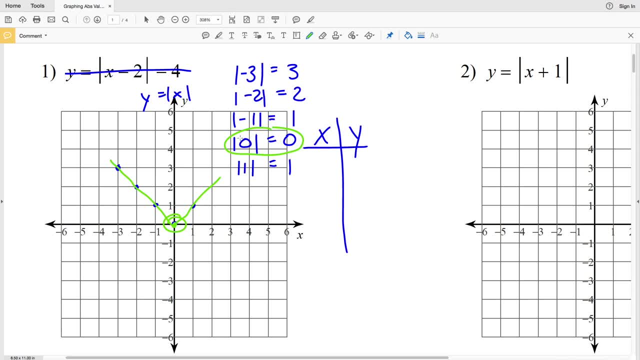 we're going to find the turning point, then we're going to find the coordinate for a number that's less than that turning point and a coordinate for a number that's greater than that turning point. So let's go ahead and start number 1, now that we have an understanding of how to graph the absolute. 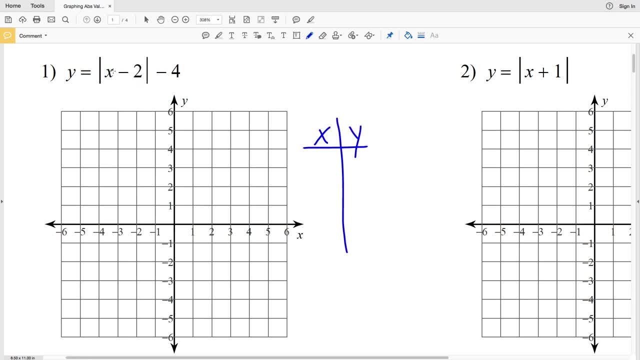 value functions. So we know that turning point occurs when the absolute value is equal to 0. So we're going to look strictly at the absolute value function. So the absolute value of x minus 2 we have to solve for when that's equal to 0. So we're looking at when x minus 2 equals 0. So we're going. 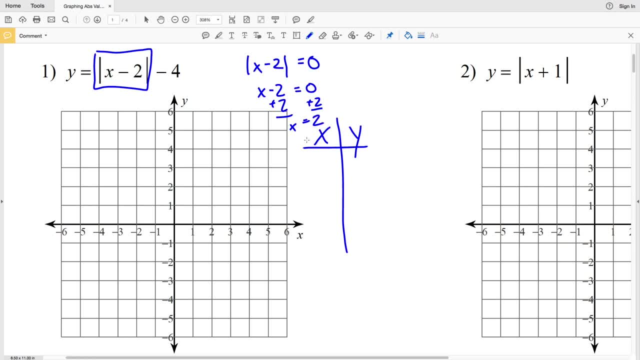 to solve for when x minus 2 equals 2.. So our turning point occurs when x is equal to 2.. Now let's plug 2 in for x and solve for y, So we're going to have the absolute value of 2 minus 2. 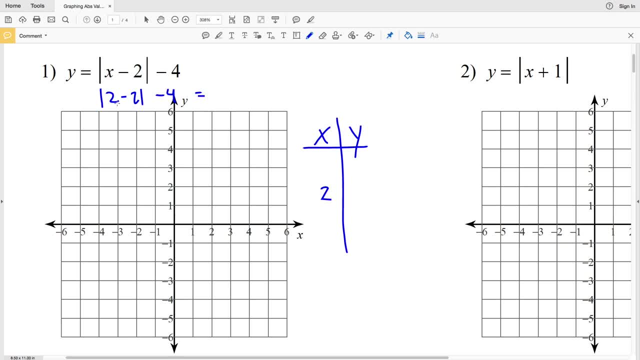 which we know is 0 minus 4.. So the absolute value of 2 minus 2 is the absolute value of 0 minus 4, which we know that the absolute value of 0 is simply 0. So negative 4 is going to be negative. 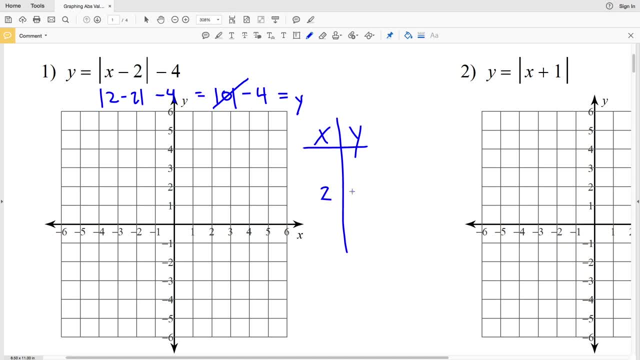 4 minus 2, and then minus 4 is going to be equal to y. So when x is 2, y is negative 4.. Now let's pick a point that's less than the value of 2.. So it's going to be to the left of our turning point. 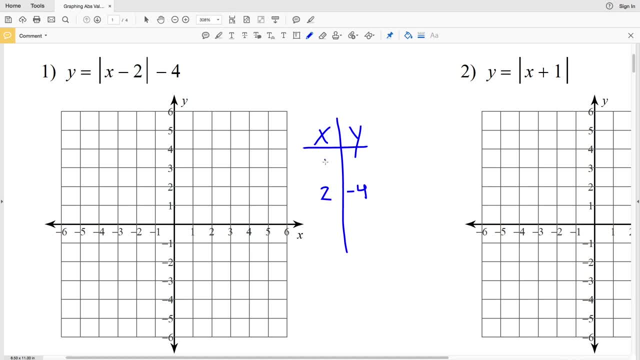 or vertex, So let's choose 1.. When x is 1, we're going to have the absolute value of 1 minus 2 and then minus 4.. The absolute value of 1 minus 2 is the absolute value of negative 1. 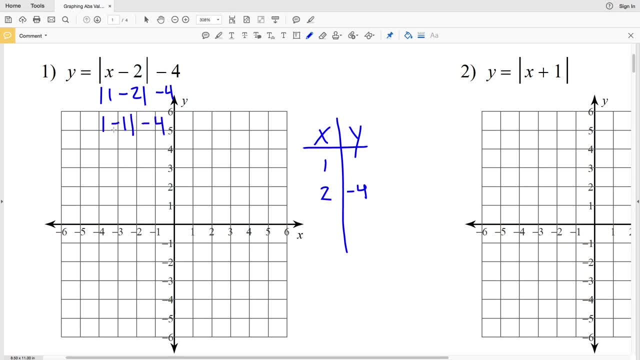 and then we're subtracting that 4.. know that the absolute value of negative 1 is a positive 1, and when we subtract 4, we get 1 minus 4, which is a negative 3. so when X equals 1, Y is equivalent to negative 3. now let's pick. 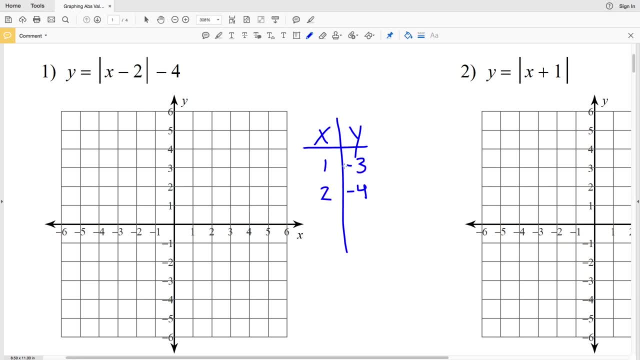 a number that's greater than 2, so it's going to be on the right side of the turning point. let's just pick 3. we're plugging in 3 for X, so we're going to have the absolute value of 3 minus 2. 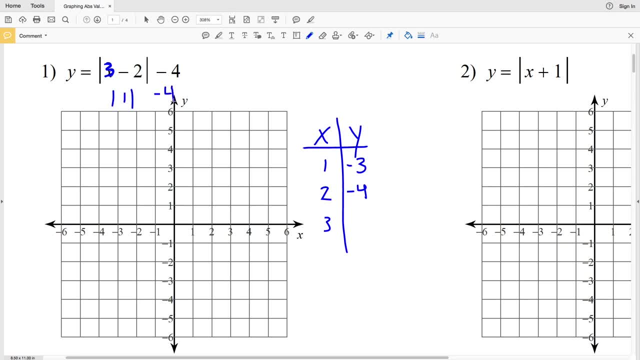 which is the absolute value of 1, and then, subtracting 4, the absolute value of 1 is simply 1. so we have 1 minus 4 and that's going to give us again a negative 3. so now we have the point 3- negative 3. so when X is 3, Y is also negative 3. 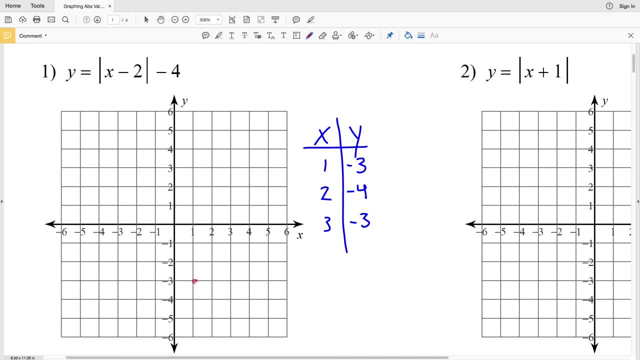 now let's plot those. we have 1 negative 3, 2 negative 4 and 3 negative 3, and just like that we'll be able to now draw our lines, starting at the turning point, drawing a positive slope, and then we'll draw the negative slope, and that's the answer to number one. also note that this: 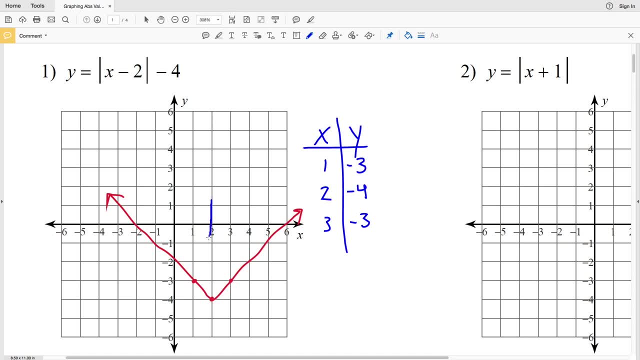 absolute value function is symmetrical. so if you were to draw the absolute value function straight down through that vertex, our points or our lines are mirrored. that's why, when we went one less than the turning point in the X direction and one greater than the turning point in the X, 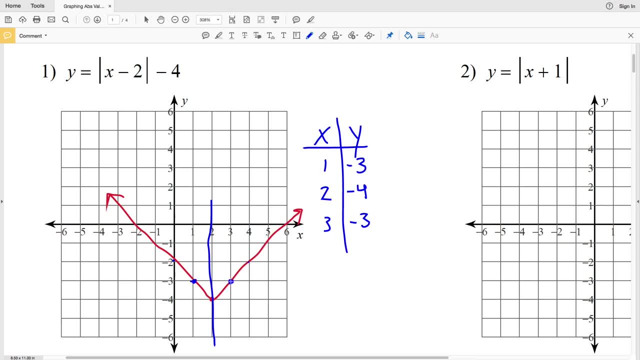 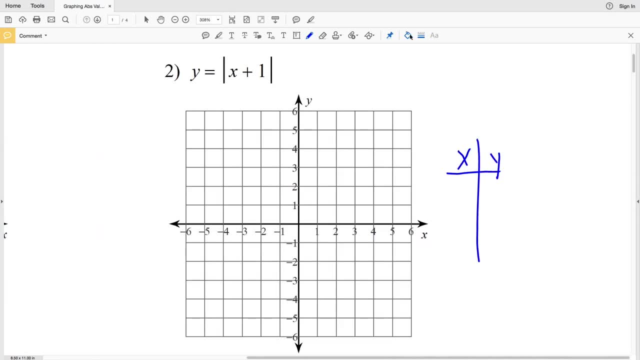 direction. our Y values are both negative. 3, let's go ahead and move on to number 2. set up our XY T table and we're going to solve for that turning point. so that's when what's inside the absolute value function is the absolute value function and the absolute value function is the negative. 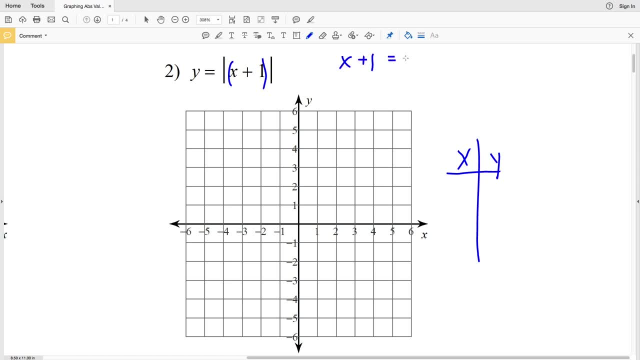 is equal to 0. so X plus 1, when does that equal 0? we're going to subtract 1 from both sides to get the X equals negative 1. so when X is negative 1, whatever our y value is that's going to be our. 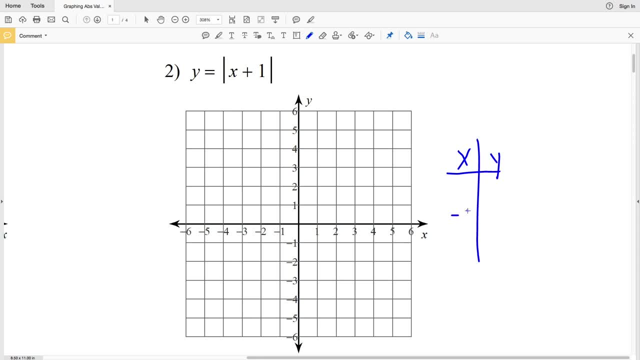 vertex. so we'll write negative 1 and I like to put it in the middle of my t-table. so I know that I need to do a point that's less than that negative 1 value and a point that's greater than that negative 1 value. so let's go ahead and plug in negative 1 for X. so when we plug in negative 1, 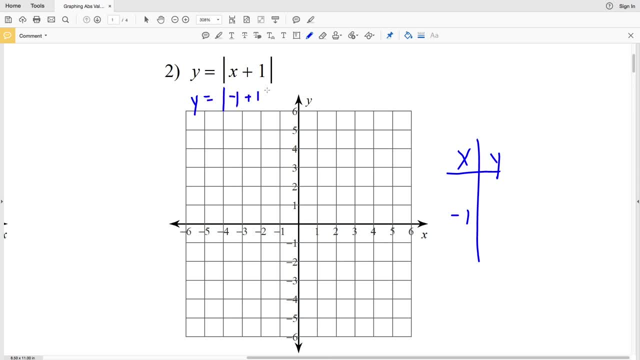 we get that y equals the absolute value of negative 1 plus 1, which we know is y equals the absolute value of 0, which is 0. so when X is negative 1, Y is 0. now I'm going to do one unit less than the turning point in the X. so I'm going to choose negative 2 and 1 greater than the vertex. 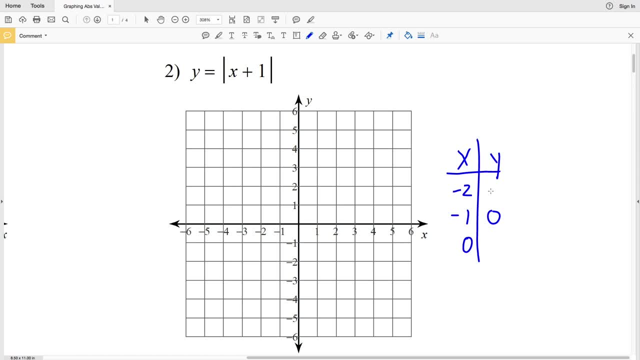 X coordinate 0. so now, if you remember, we talked about the absolute value function being symmetric. since negative 2 is 1 less than negative 1 and 0 is 1 greater than negative 1, those two should have the same y values. let's check it out. so if we plug negative 2 in for X, we get that Y is equal to the. 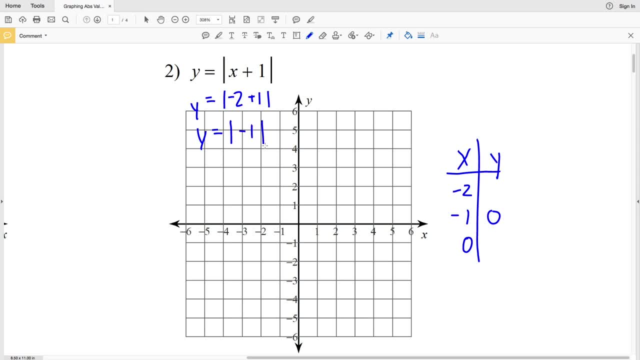 absolute value of negative 1. so Y is going to be equal to positive 1. so when X is negative 2, Y is a positive 1. now let's plug in zero. when X is 0, we get that Y is equal to the absolute value of 0 plus 1, which. 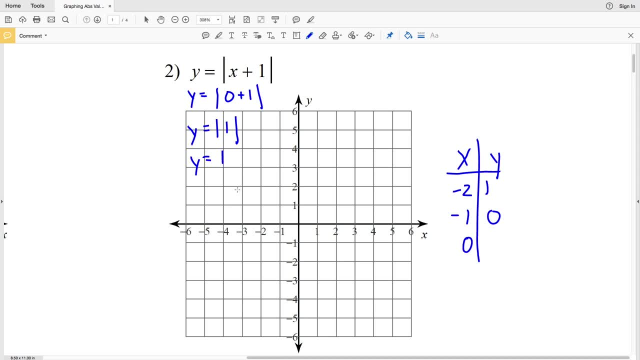 we know, is the absolute value of 1 and the absolute value of 1 is equal to 1. so when X is 0, Y is a positive one. so you can see, like I said, since it's symmetric, negative two and zero, since they're both one unit away from the turning points X-coordinate, it's negative 1 plus 1 in positive 2. 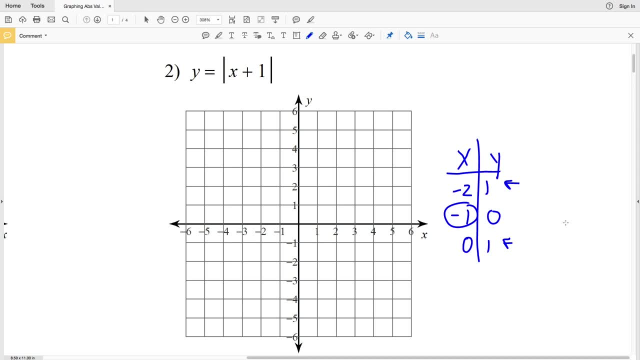 or X value. they have the same y values. let's go ahead and graph it to get our answer: negative 2, positive 1, negative 1: 0 and 0: 1. it's a straight line to the turning point and then a straight line from the turning point, and I recommend using a straight edge like a ruler or another piece of. 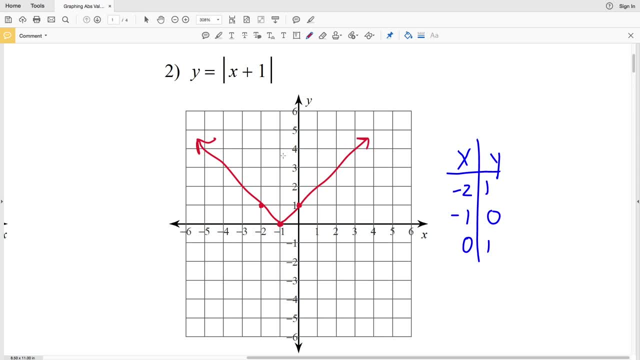 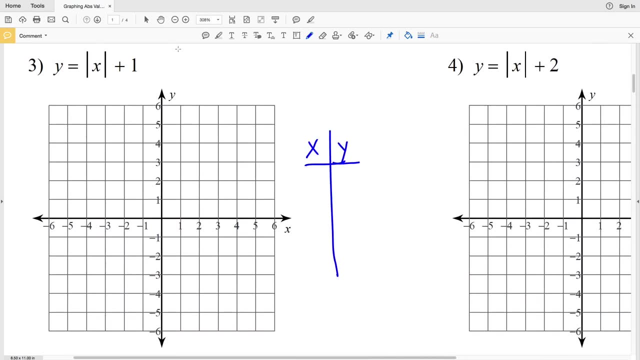 paper when drawing your lines for linear functions. let's move on to number three. again, we're going to have our T table with X and Y values. so now we're going to figure out our turning point. the turning point occurs when what's inside the absolute value quantity is equal to 0, so that 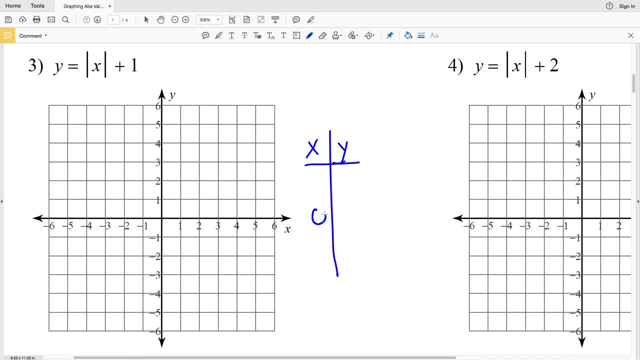 occurs when X is 0. when X is 0, our Y is a positive 1, since Y equals 0 plus 1, which is simply 1. now I'm going to choose a point that's less than the X value, so negative 1, and I'm going to do a. 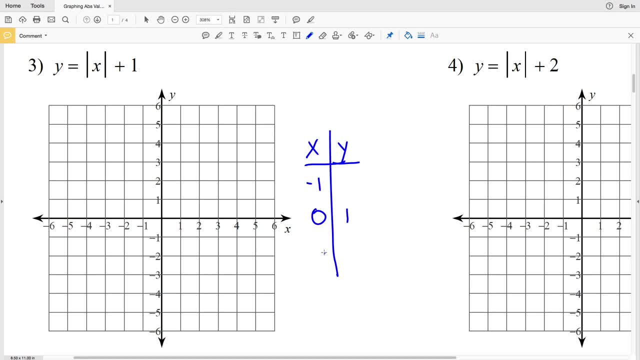 point that's greater than the X value of 0, so a positive 1. when we plug in negative 1, we get that Y equals the absolute value of negative 1 plus 1. so that's going to be: Y equals positive 1 plus 1. 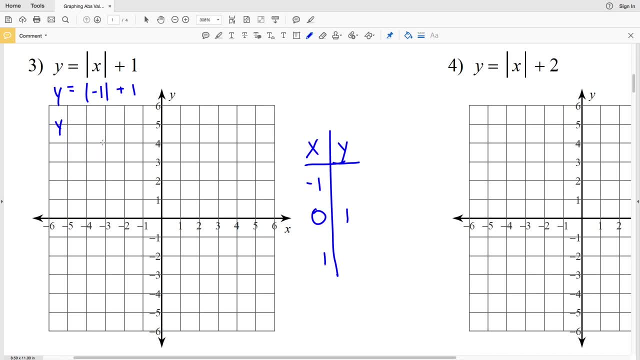 so Y is equal to 2. so an X is negative 1, Y is a positive 2. now let's plug in a positive 1. if we plug in a positive 1 for X, we get the absolute value of 1 plus 1, which we know is 1 plus 1, which will give us 2. so an X is positive 1, Y is a positive 2 now. 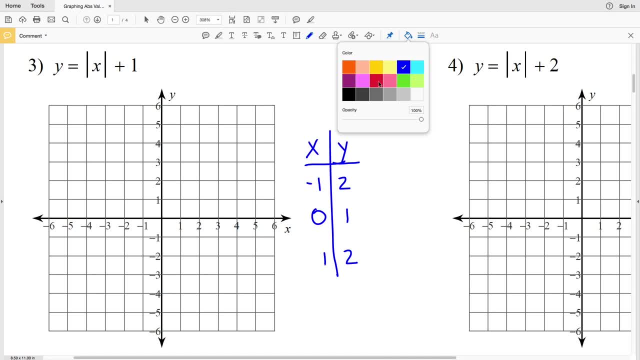 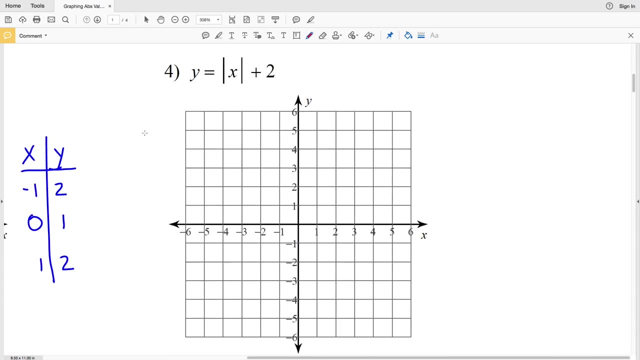 we have three points, including our turning point. so let's go ahead and graph this negative: 1, 2, 0, 1 and 1, 2, and that's the answer to number 3. moving on to number 4, again with the T table, we're going to.